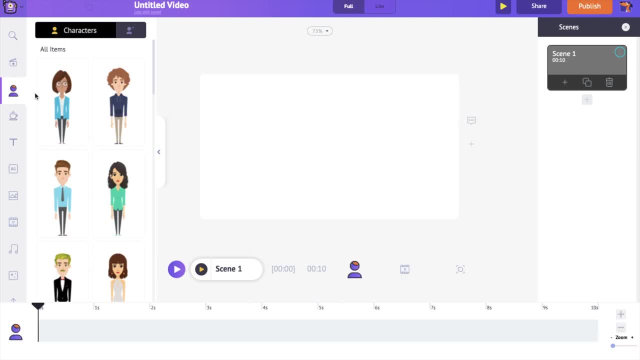 have a video and audio timeline And the last one is the camera timeline. On the left hand side is the library. It has different elements like animated characters, properties and music tracks that you will need to create a video And, the best thing is, all these assets are copyright free. 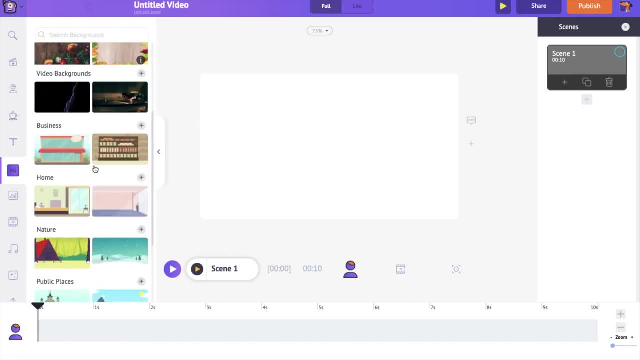 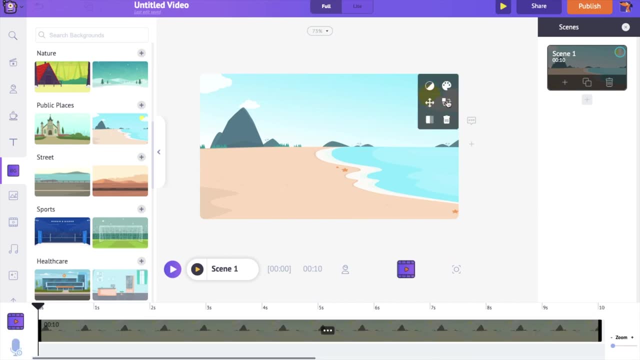 Let's start with adding the background to the scene. Go to the background section of the library and select a background. If you further click on the background on the workspace, you can see a set of options. This is the item menu of the background. Any element added. 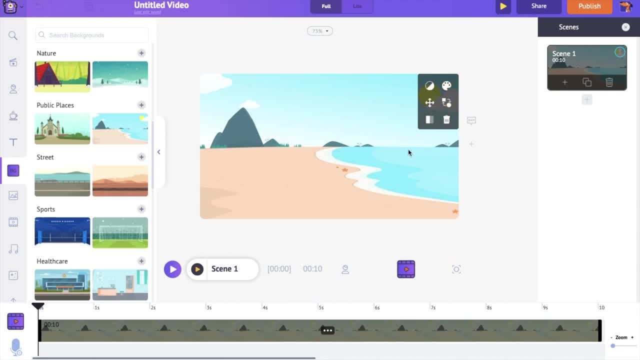 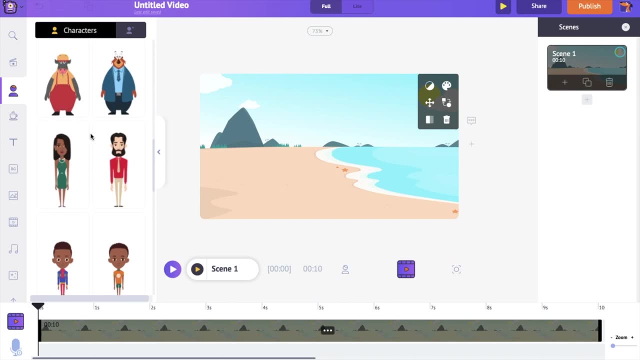 to the workspace will have an item menu. These options let you further edit the background. Now I want to add a character. Let's add a kid character that is walking in the background. Open the character section of the library. Let's select this one. 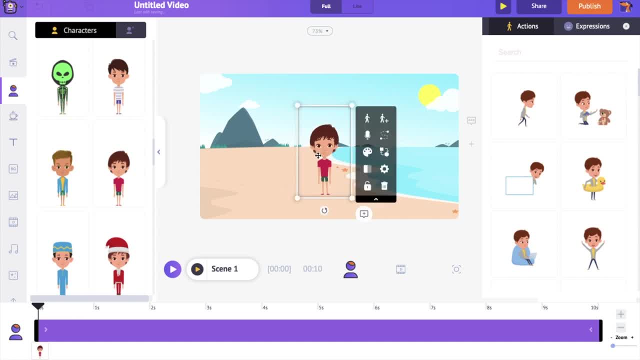 Let's add a character. Let's add a character. On the right hand side you can notice the action step. From here you can select among 500 different actions. I want the character to be walking a dog. You can see that the 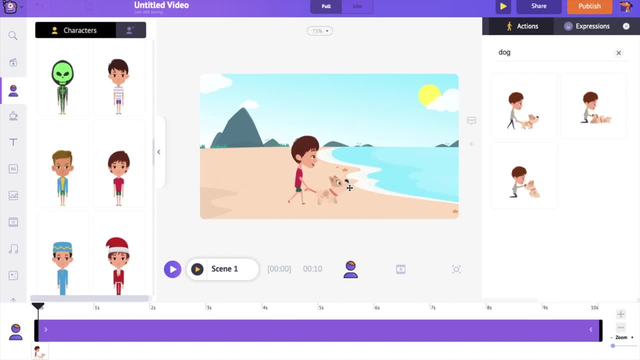 dog and the sand are almost the same color, So let's change the color of the dog to improve its visibility. You can change the colors of the character using the change color option present in the item menu of the character. On the timeline. you can notice a purple colored bar. You can notice this bar for any kind. 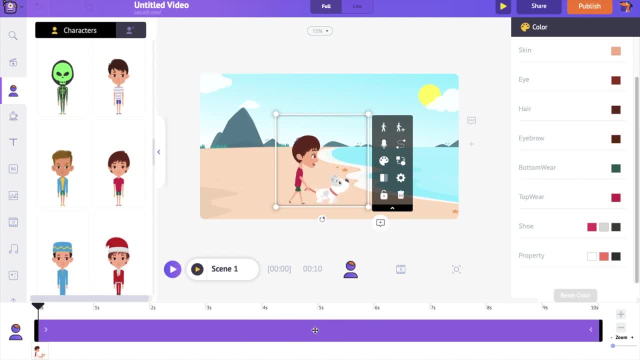 of property or object added to the scene. It represents the duration for which this character is going to be visible. For example, if I want the character to appear a little later, let's say after the third second, I'm just going to drag the left edge of the bar. 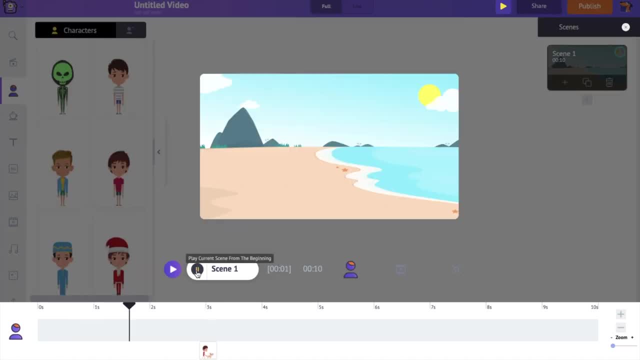 and keep it around the third second. So now, if I preview the scene, you can see that the character is visible only after the third second. So, like this, by adjusting this purple bar, you can control the visibility of any element added to the scene. Right now, the 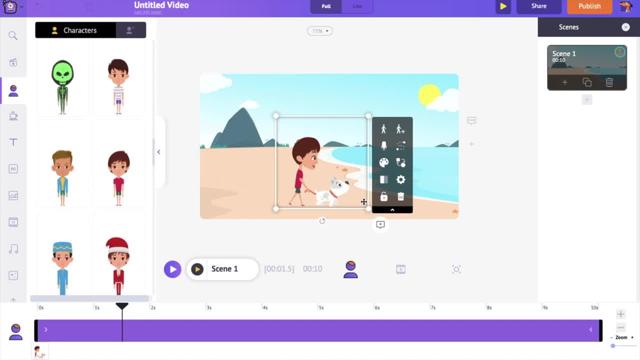 character looks like walking in the same place. Let's see how to make it move between two different points. I want the character to enter the scene from the left and leave on the right side. Let's keep the character on the left side of the scene. On the item. 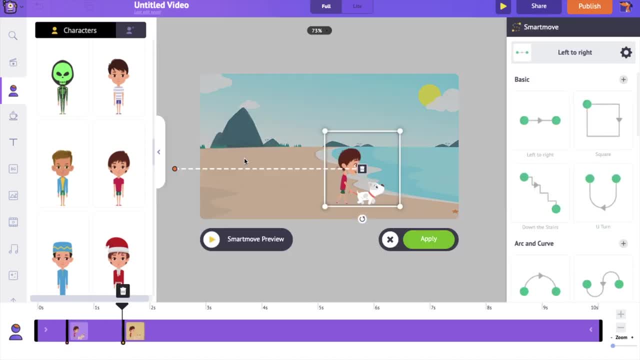 menu of the character there is an option named smart move. Click on it. So this is the position two of the character. Let's keep it on the right side. The character will be moving from the position one to two On the timeline. you can notice two thumbs. They. 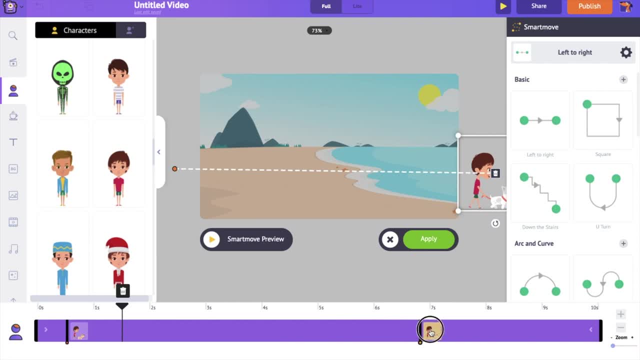 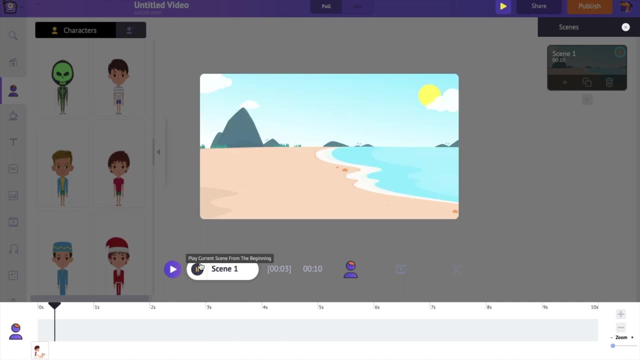 represent the position one and two of the character. You can control how much time the character is going to take between the two positions using these thumbs over here. Let's make the character enter the scene around the third second and exit the scene around the eighth second. Let's preview the scene. So this is how you can move a character from. 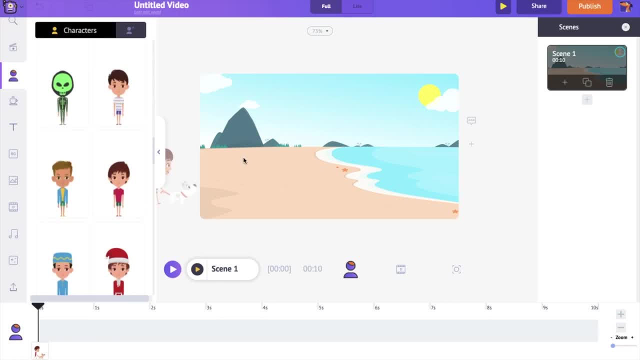 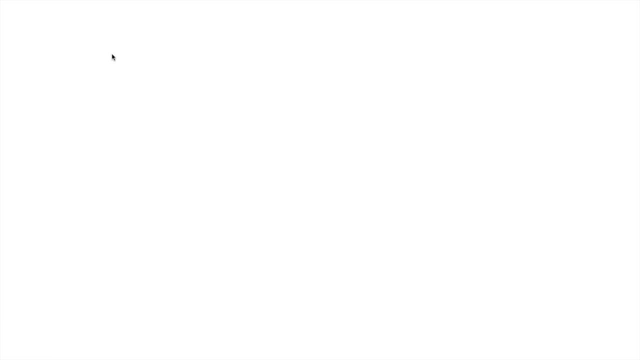 one place to another. Let me add the main character, to which we'll be adding the voiceover Instead of using the character from the library. this time we'll be using the voiceover, So this time we'll create a custom character. Open the my characters section and select. 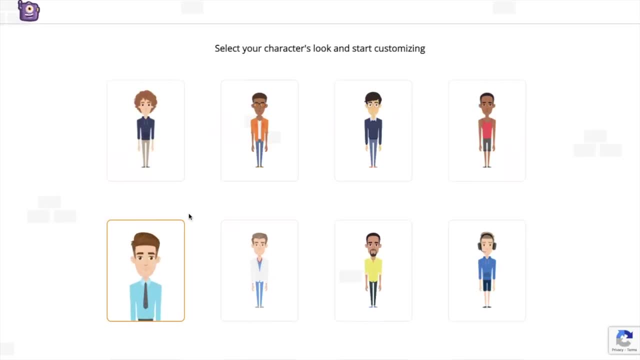 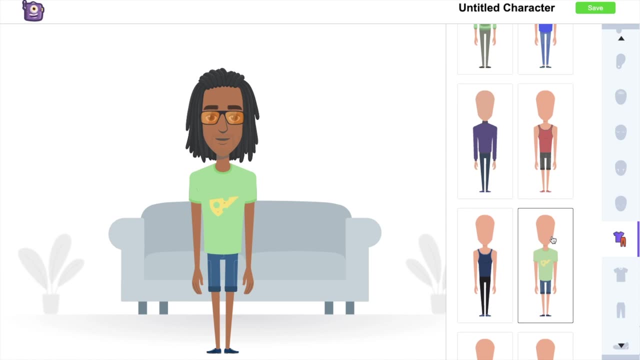 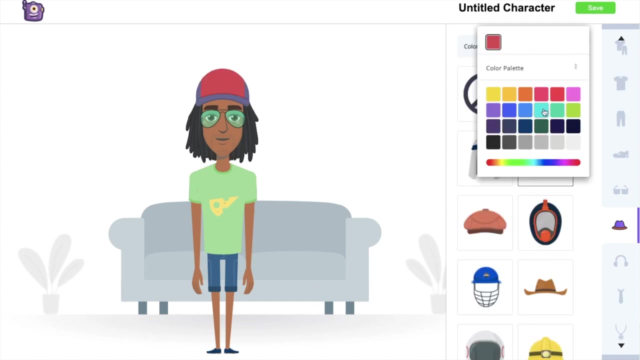 the create your own option. Now select the gender and the basic template and start building the character. You can change the facial features, attire wearables. You can create billions of unique characters using all these options. Finally, you can save the character using 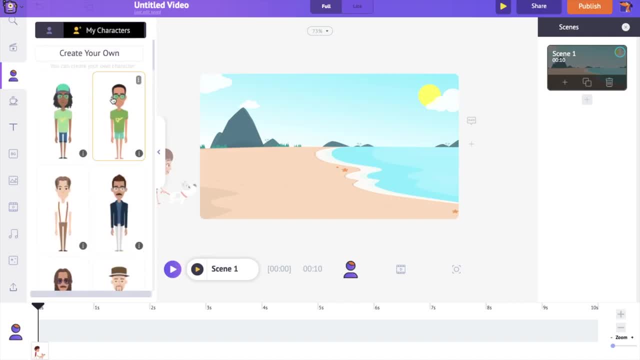 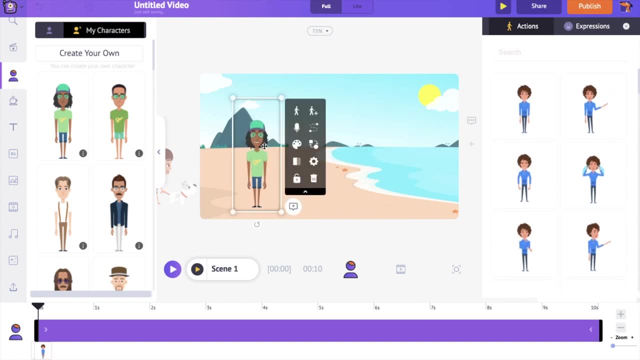 the option over here. Now get back to the video project and you can find the newly created character under the my characters section. Click on the character. I want this character to walk into the scene and then it should wave towards the viewers and talk. So the character has to do three different actions. 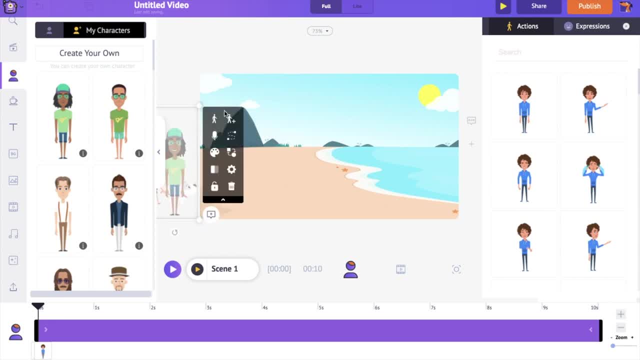 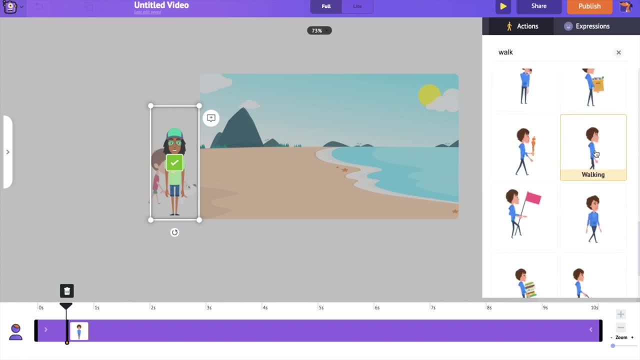 walking, waving and then talking. To add multiple actions to the same character, use the action plus option from the item menu. Now edit the action. To add the next action, click on the plus option on the right hand side On the timeline position. the actions at the right. 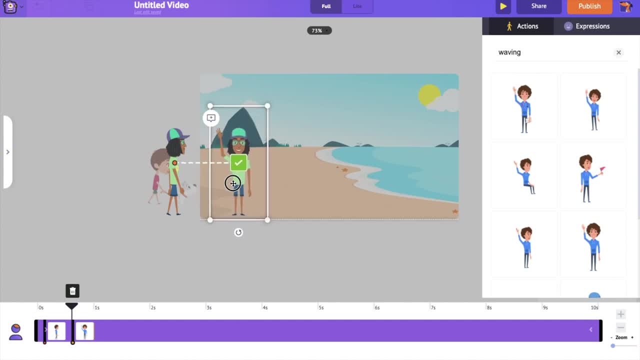 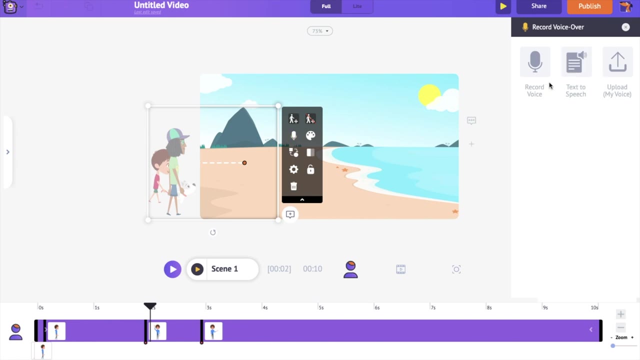 time. Let's make the waving action appear after 2 seconds and the talking action at the third second. Let's see how to add the voiceover. Go to the item menu and click on the add voice option. Now you have three different options to add the voiceover. Click on this blue icon record. 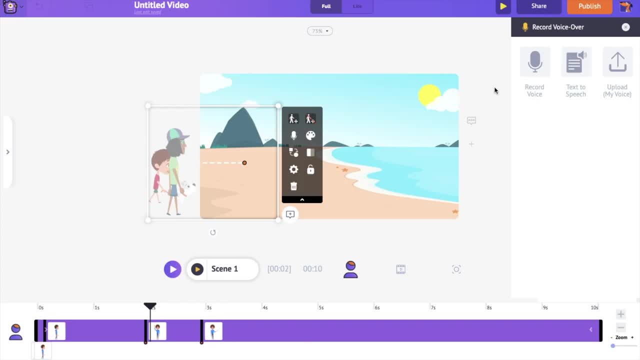 your voice and add it to the video. The last one is the upload option. You can add any pre-recorded audio files as a voiceover using this option. The second option is the text to speech option. For this video, we are going to use this one. 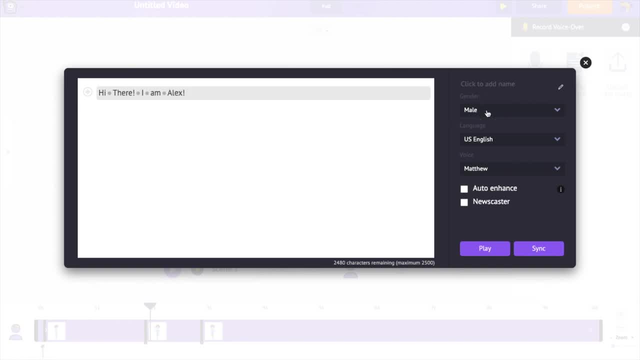 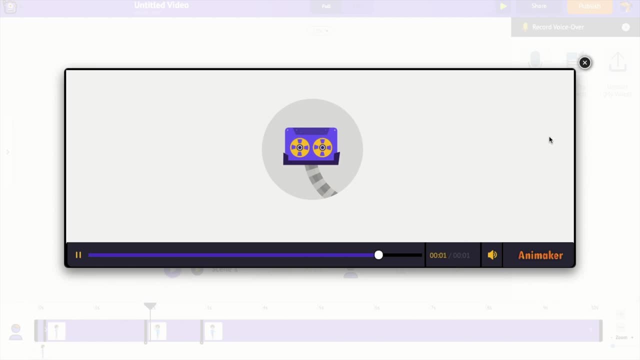 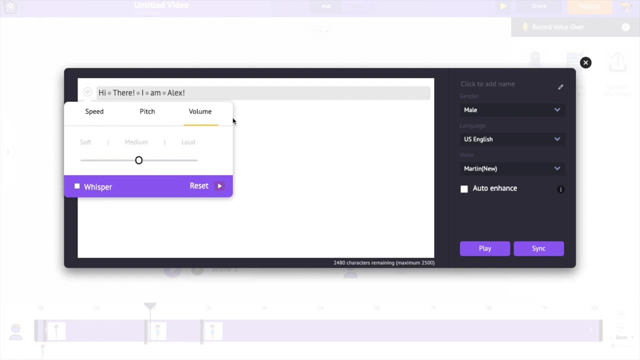 Just type in the dialogue, select the gender, language and voice. Right now the voice sounds a bit robotic, but you can use the options over here to improve it. You can control the speed, pitch and volume. You can also add pause and breathing effects. 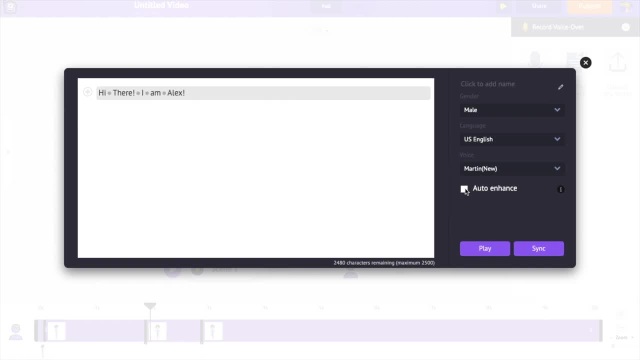 between words. If you are a paid user, you can easily use this auto enhance feature to control the speed, pitch and volume. You can also add pause and breathing effects between words. If you are a paid user, you can easily use this auto enhance feature to control the speed pitch. 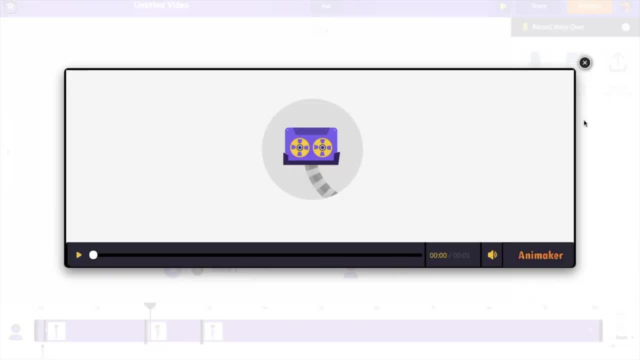 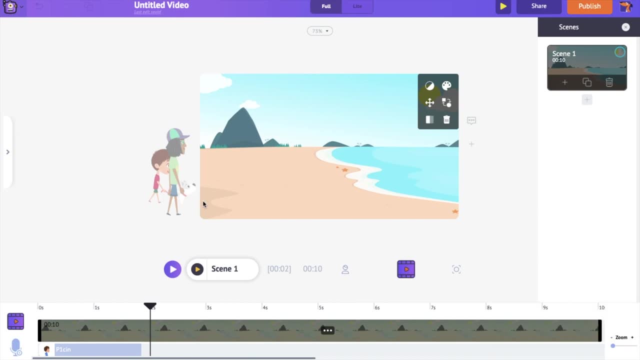 and volume To enhance the voice. select the sync option to add it to the video. Now, on the audio timeline, you can notice the voiceover track. Let's adjust its position in the timeline to match it with the actions that we added earlier. 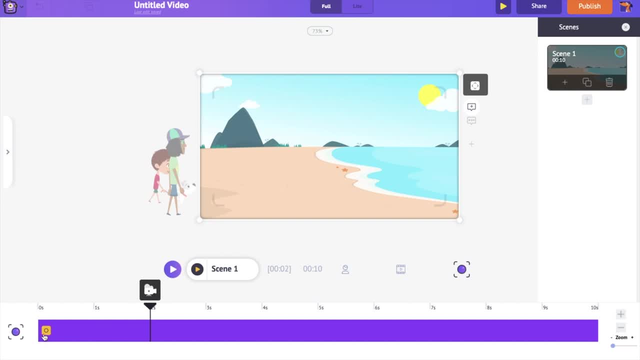 Let's see how to add camera effects. Open the camera timeline. There are two camera options: static camera, dynamic camera. To apply the camera effect, select the dynamic camera option On the timeline. you can see a new pink colored part. This is the duration for which this dynamic camera effect is going. 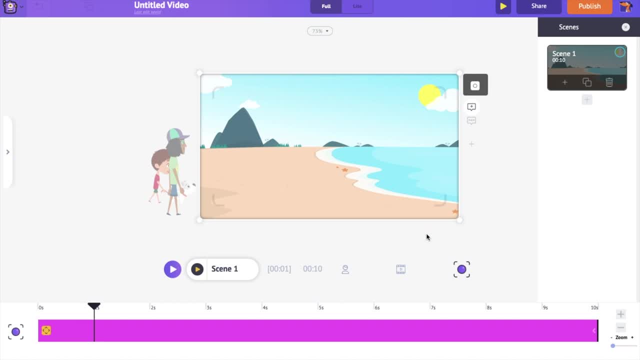 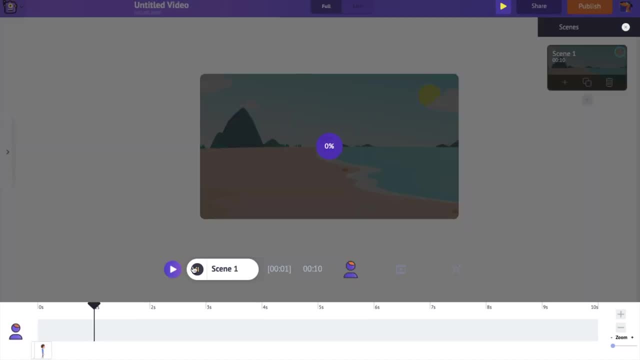 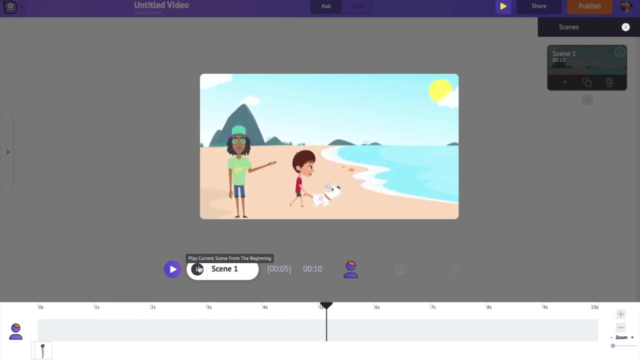 to happen. Drag it and keep it till the duration you want it to happen. Now, on the workspace, adjust the camera's frame and keep it where you want it to be focused. Let's preview the scene. If you want to add music to the video, go to the music section in the library Here. 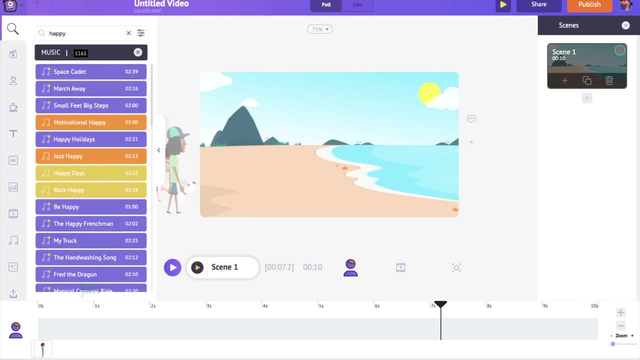 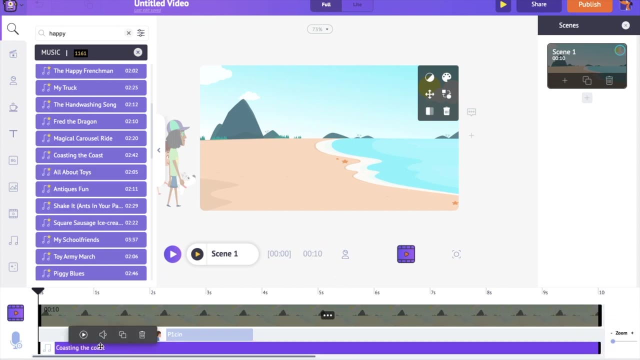 you have more than 30,000 music tracks. To have a preview of a track, keep the pointer over it And click on a track to add it to the video. Now you can notice the music track on the audio timeline If you further click on the. 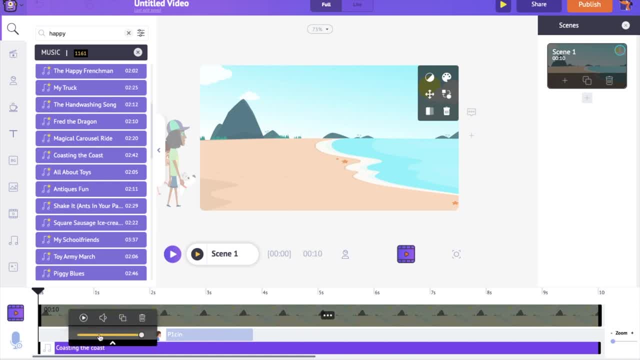 music track, you will get a few more options. Let's reduce the volume of the track so that the music won't overpower the voiceover track. Hi there, I am Anirudh. In this video, I am going to show you how to add a music track. 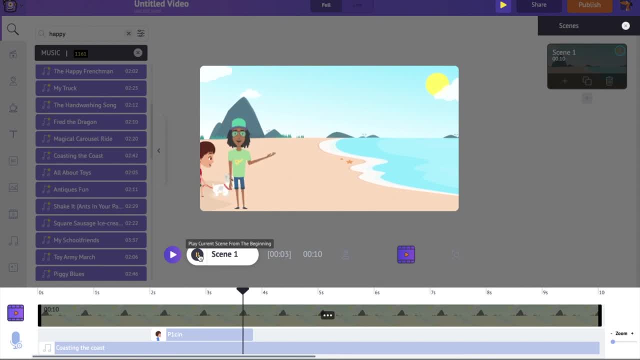 to your audio timeline. To add a music track to your audio timeline, go to the music section in the library. Here you have more than 30,000 music tracks. To have a preview of a track, keep the pointer over it. Hi, there, I am Alex. 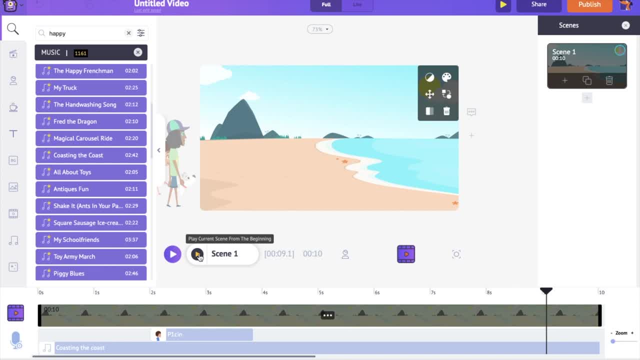 In the same way, you can create multiple scenes. Click on the add scene option in the scene section to add a new scene. You can delete a scene using the option over here To download the video. select the publish option at the top. click on the download video.